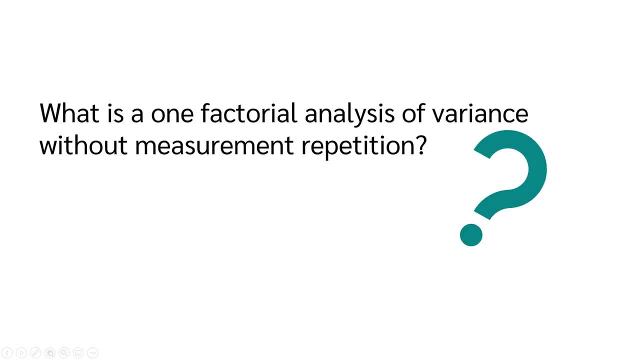 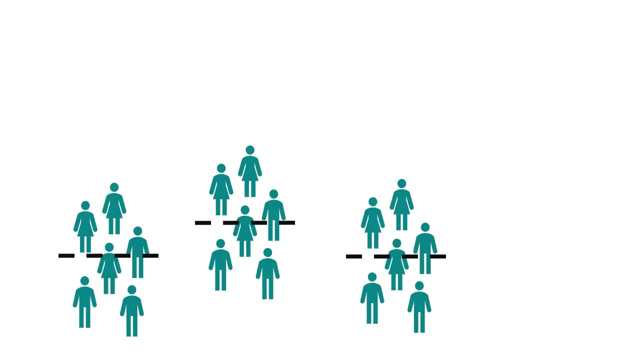 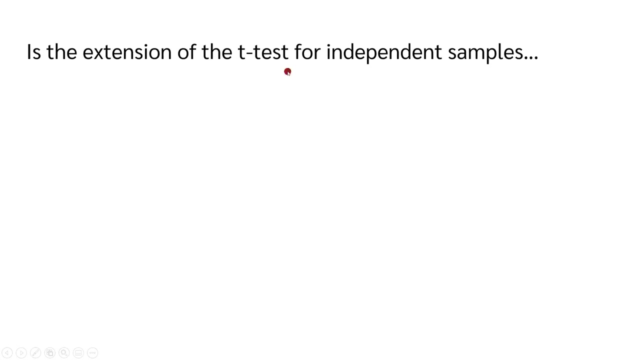 repetitions, And that's where we start. The first question is: why do you need an analysis of variance at all? What does an analysis of variance do? An analysis of variance checks whether there are statistically significant differences between more than two groups. Therefore, the analysis of variance is the extension of the t-test for independent 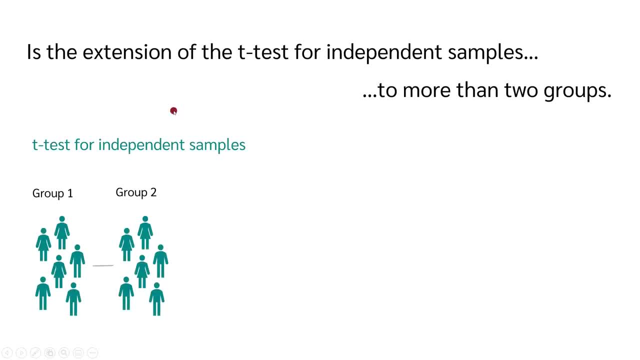 samples to more than two groups. When calculating an independent t-test, we looked at whether there is a difference difference or, more precisely, a difference in means between two independent groups, For example, if there is a difference in the salary of men and women. In this case, we have two groups. 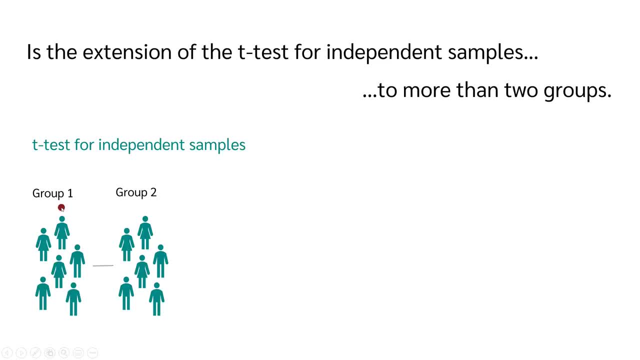 the men's group and the women's group. If we want to compare more than two independent groups, we use the analysis of variance. In case of the t-test, we used an independent t-test if the two groups or samples were independent. This is the case if one person in the first group 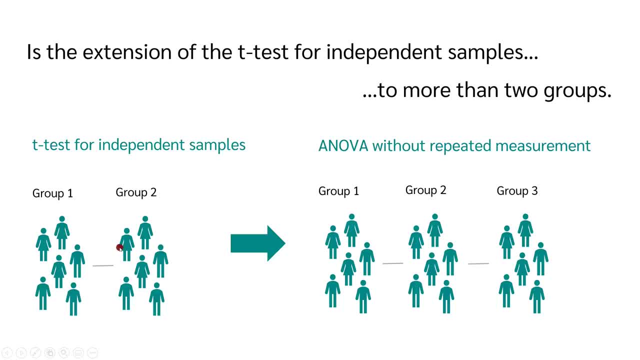 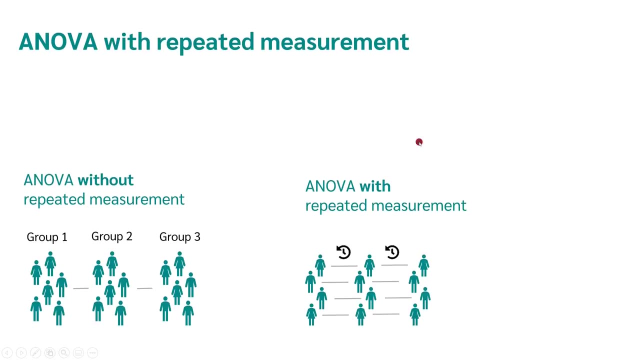 has nothing to do with a person from the second group. Exactly the same now applies to the analysis of variance without repeated measures, Except that here we have at least three independent samples. If we have more than two dependent samples, we would use an analysis of variance with. 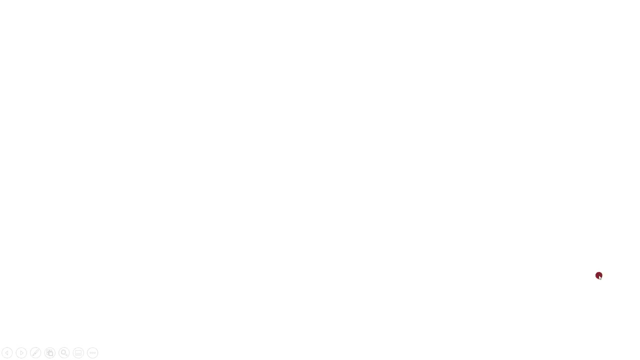 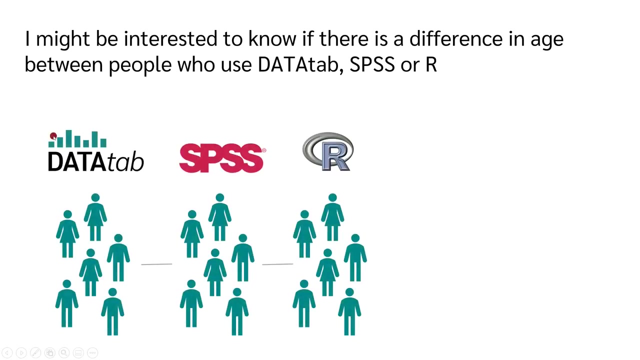 repeated measures. Now let's look at an example. Let's say that, as the founder of Datatab, I might be interested in whether there are differences in the age between people who use Datatab, SPSS or R. In order to do this, I take a sample of people who use statistical software. 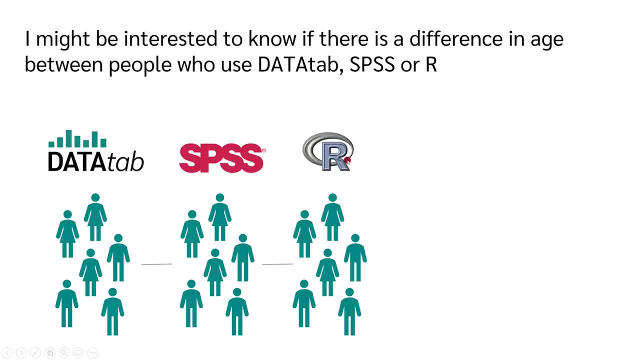 and ask them which statistical software they use and how old they are. I've only compared three groups in this example. Of course, there could also be more groups. In order to analyze this example, I would now use an ANOVA. So the next question is: what is the research question? I can answer. 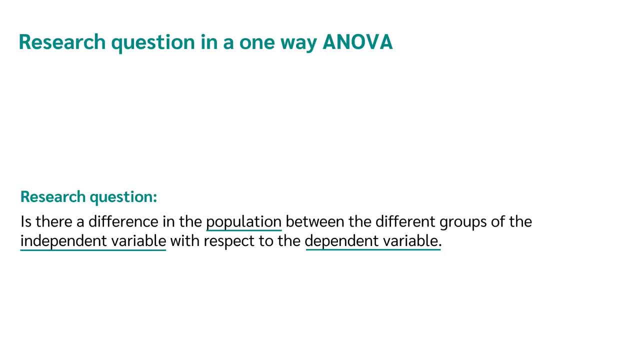 with using an ANOVA. The research question is: is there a difference in the population between the different groups of the independent variable in relation to the dependent variable? The independent variable is the variable with the different categories. In our example it is the statistic software used. Here we 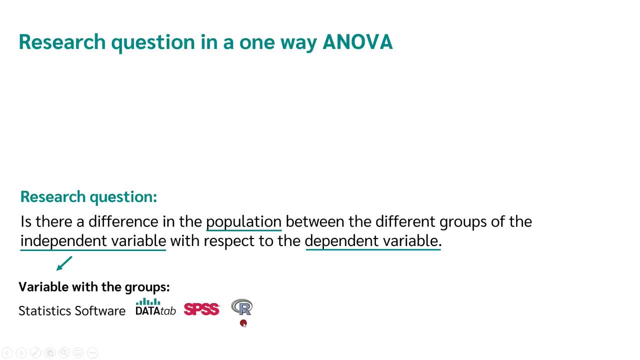 have the three groups Datatab, SPSS and R. The dependent variable in our example is the age of the software users. We would like to know whether the groups of the independent variables have an influence on the dependent variable. Of course, the analysis of variance does not give us any information about the direction. 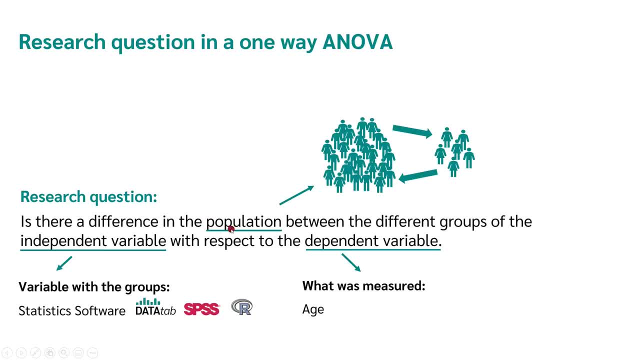 of the causal relationship. But why is our research question about the population? Don't we just have a sample? Actually, we want to make a statement about the population. Unfortunately, in most cases it is not possible to survey the whole population and we can only draw. 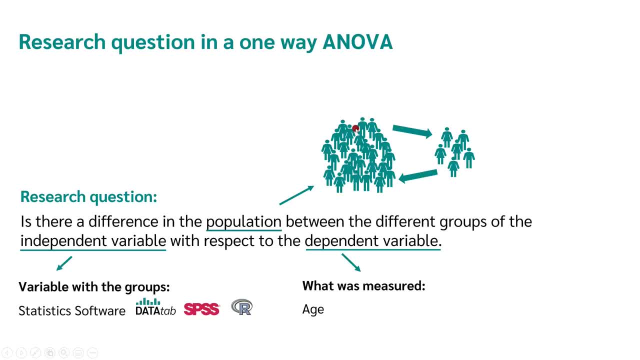 a sample. The aim is to make a statement about the population based on our sample, with the help of the analysis of variance. For our example, the question would be: is there a difference between the users of different statistical software solutions in terms of age? 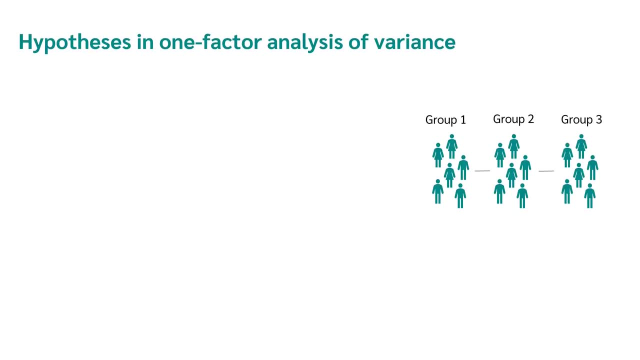 But what about the hypotheses? In the case of the analysis of variance, the null hypothesis is that there are NO differences between the means of the individual groups. We have our individual groups, of which we can calculate the mean in each case. Our null hypothesis is that there. 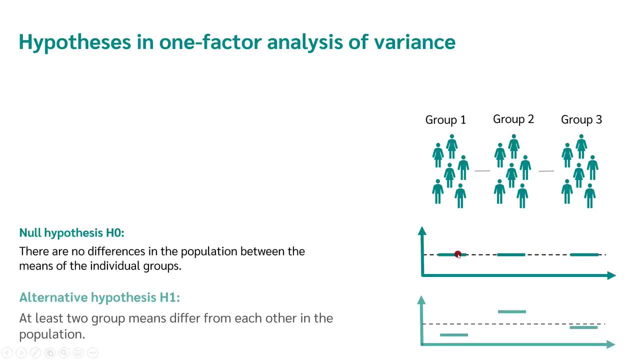 is NO difference in the mean, in the mean in the the mean in the population. The alternative hypothesis H1 is that there is a difference between at least two group means. Therefore our null hypothesis assumes that there is no difference and the alternative hypothesis says that there is a difference. All well and good. now we know. 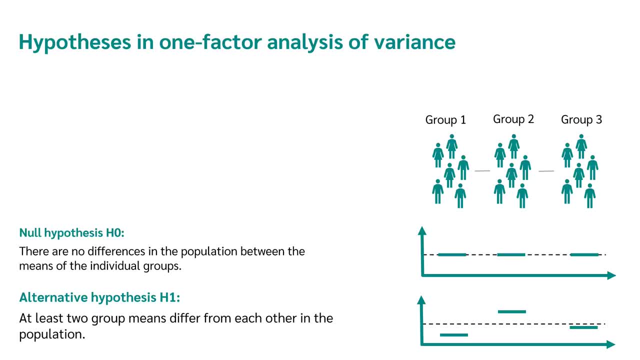 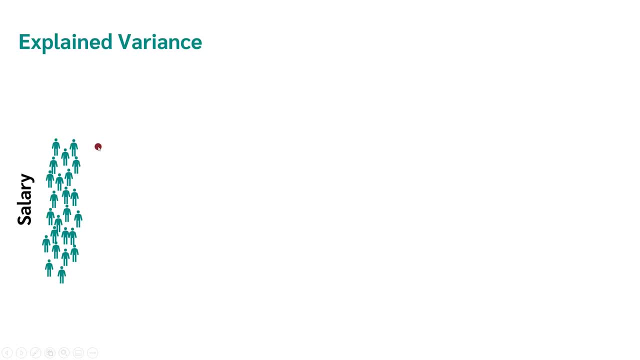 what the null hypothesis is. But what does this mean graphically? How can one picture that vividly? Let's say we want to test whether there is a difference in salary between the three groups, group one, group two and group three. The salary has some dispersion. Some people earn 400 euros a 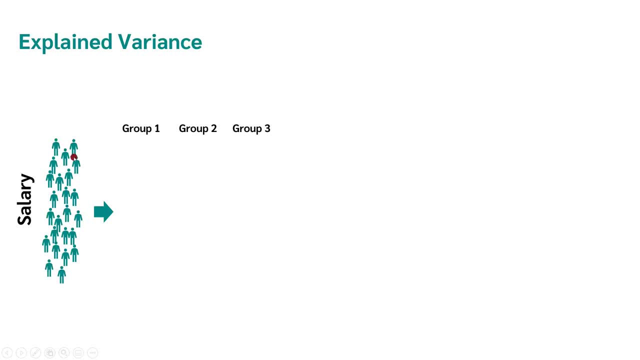 month, some 2 600 and others 6 000 euros a month. Thus, both in the population and in our sample, the salary is broadly distributed. Now the question is: where does this vanish? Let's say we want to test whether there is a difference between the three groups. group one: 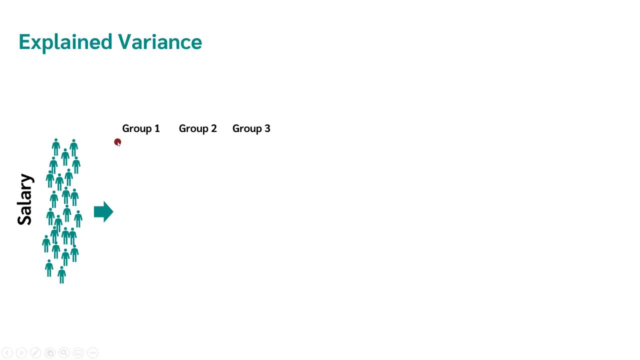 variation come from And can we explain some of the variation by these three groups? So how much of the variation in salary can we explain by dividing the people into these three groups? In the extreme case, the result could be that the salary in group one has this distribution. 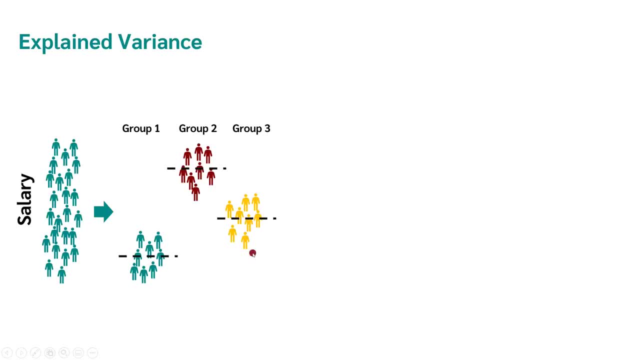 in group two that distribution and in group three the distribution would look like this: In this case, the division into groups could explain a lot of variance in the variable salary. The result would be different in this case. Here, however, we could explain almost no variance by 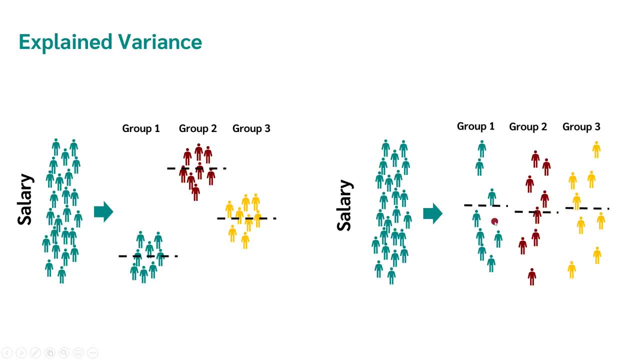 forming the three groups. Within the groups, the variance is almost the same as in the whole sample. Therefore, it does not matter whether we form the groups or not. The three groups have nearly no influence on the salary. If we now look at the variance within the groups, we can see that 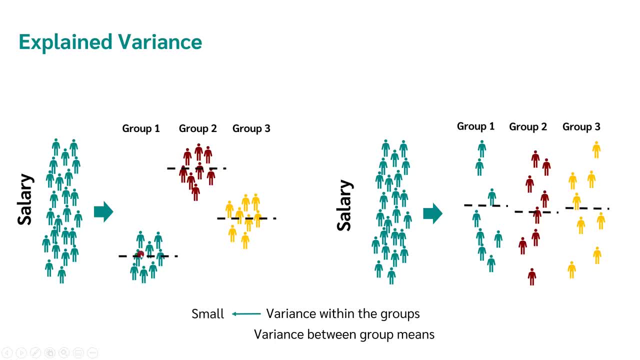 in this case we have very small variances within the groups. So within this group we have a very small variance, Within that group we have a small variance, And also in the last group. On the other hand, the variance between the groups is very large because the mean values of the 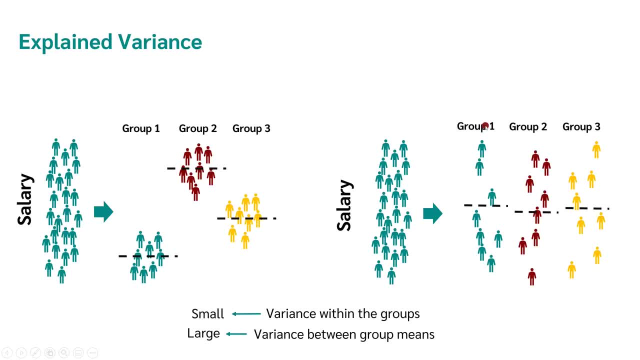 individual groups are very small. So if we take a look at the variance within the groups, we can are very far apart. In the other case, we have a very large variance within the groups. However, the variance between the groups is very small because the mean 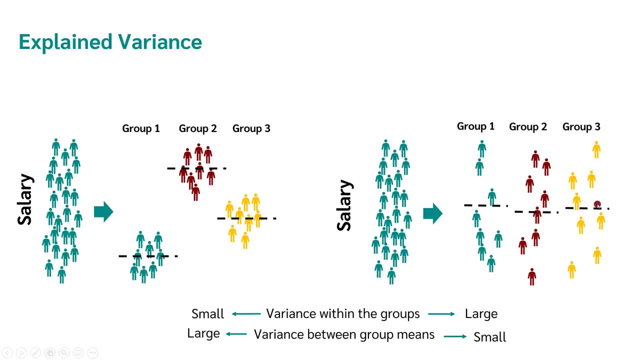 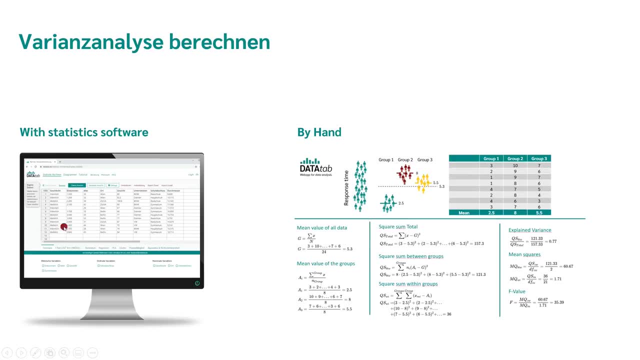 values of the groups are very close together. How can we calculate an ANOVA? There are two possibilities for the calculation. Either you use a statistics software like Datatab or you calculate the analysis of variance by hand. Admittedly, no one will calculate the analysis of variance by hand, but the